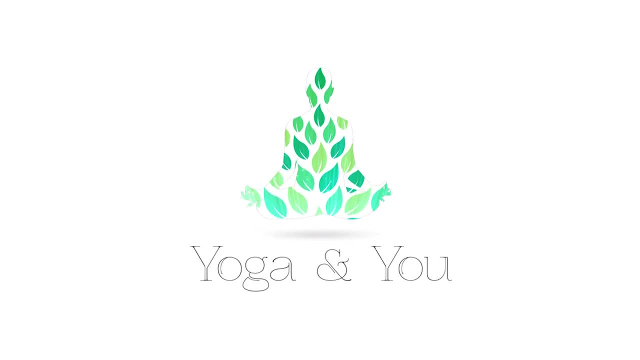 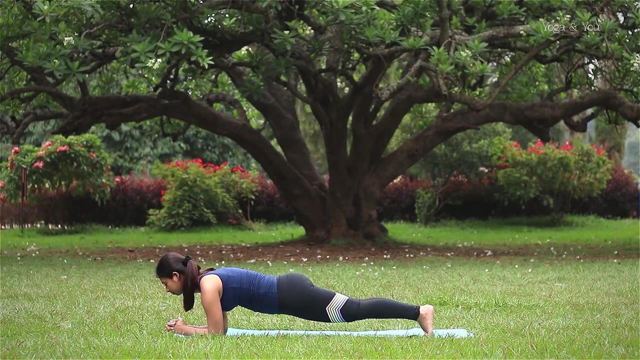 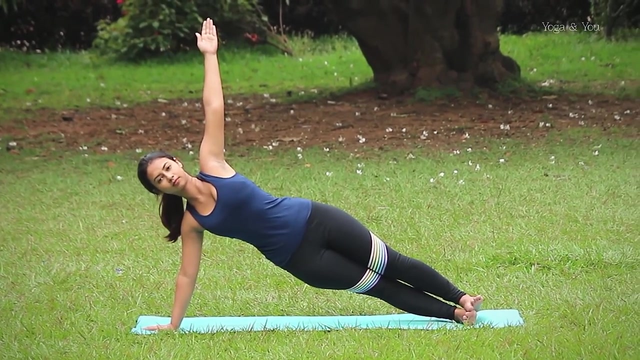 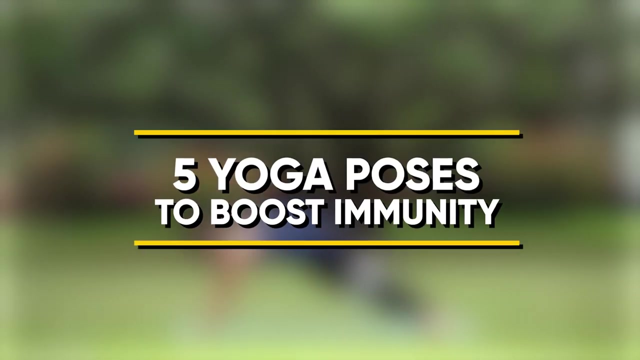 A stronger immune system means better chances of fighting through and overcoming any disease. Apart from a healthy diet and nutritional supplements, yoga can also boost your immunity by reducing psychological stress, increasing blood circulation and enhancing breathing. Here are 5 yoga poses that will help you boost your immunity. 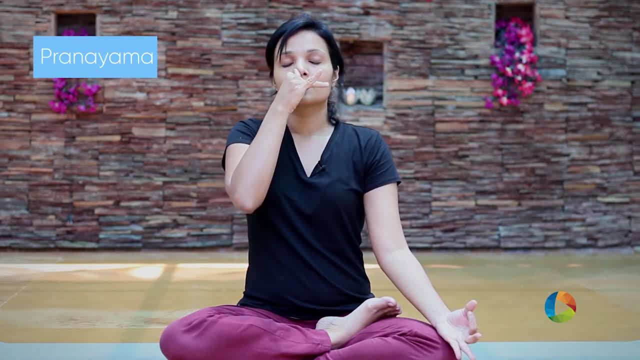 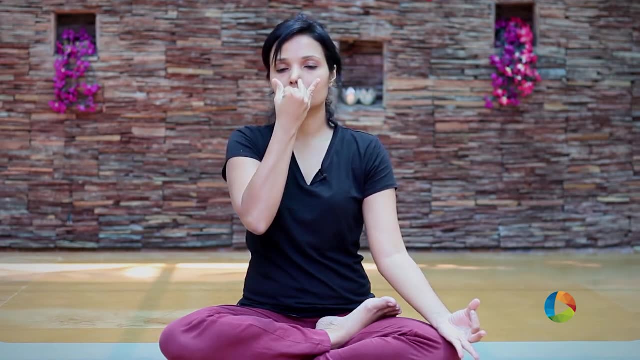 Pranayama, or Deep Breathing. Pranayama helps in reducing stress hormones and calms down the nervous system, which in turn supports in making a healthy immune system. Pranayama also conditions and maximizes the lungs breathing capacity, along with activating 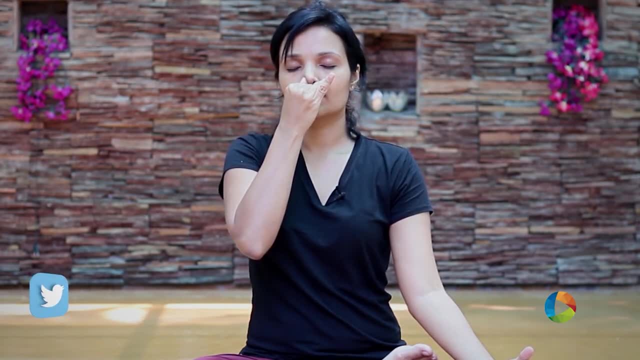 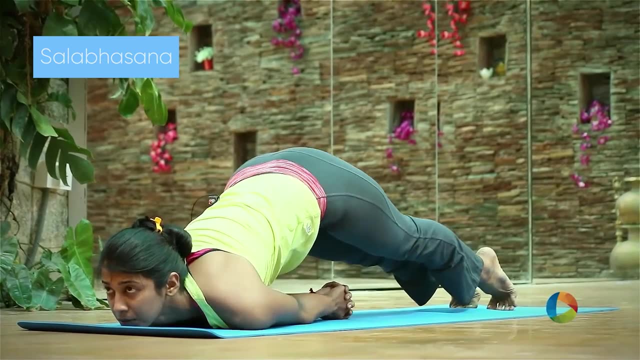 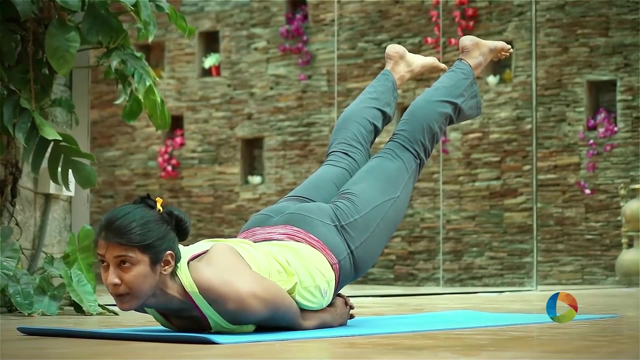 the lymphatic system. Regular practice will increase overall resistance. Salabhasana or Locust Pose: This pose involves lying down on the stomach and lifting the legs, While pushing the arms behind. this process helps in increasing the blood circulation to your intestines and rectal muscles, which is important for better digestion and a stronger 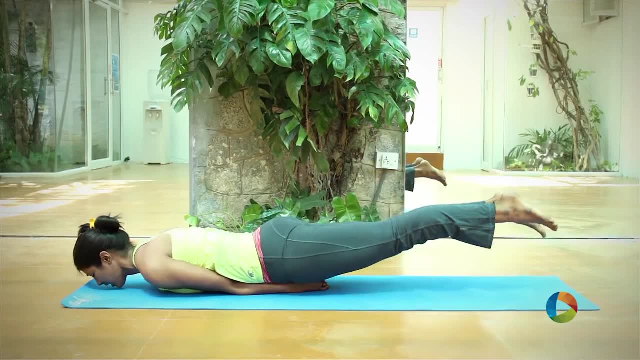 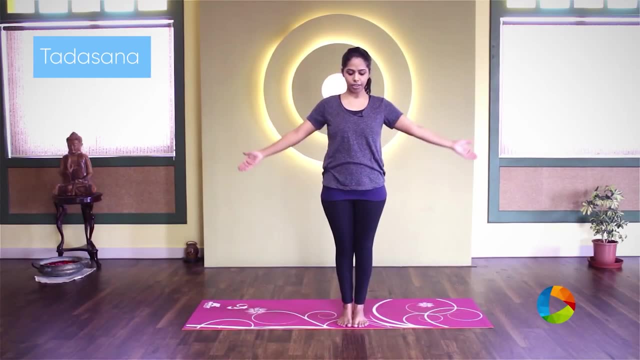 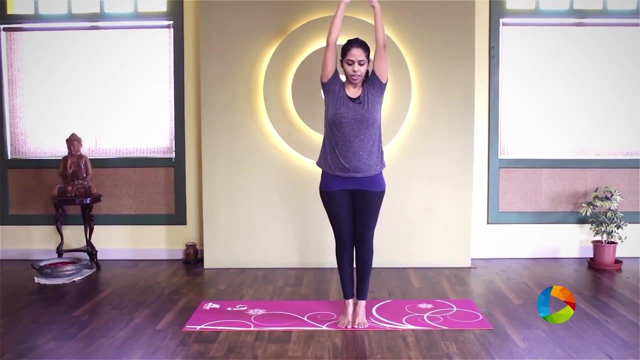 immune system. This pose also alleviates back aches caused due to prolonged working hours. Tadasana, or Mountain Pose: This asana is an easy pose that can help develop a better immune system. The asana helps in correcting your posture and strengthening your spinal column. It can also improve your mental awareness. 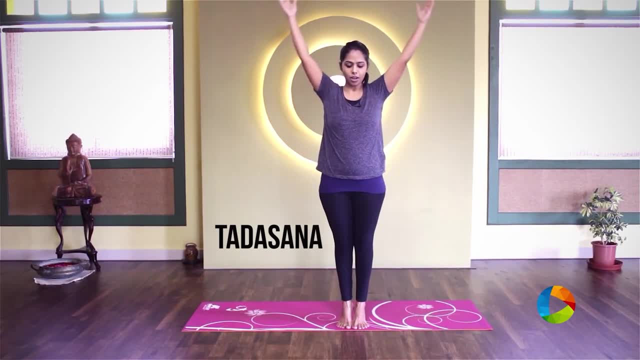 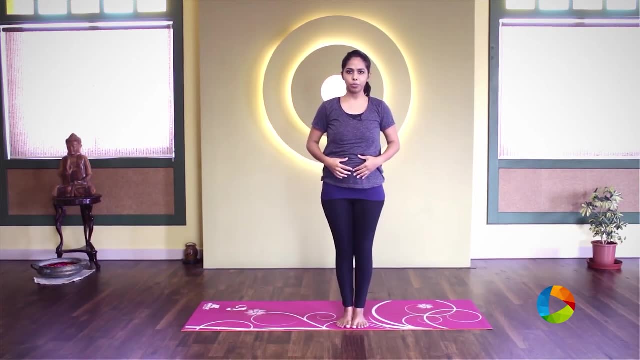 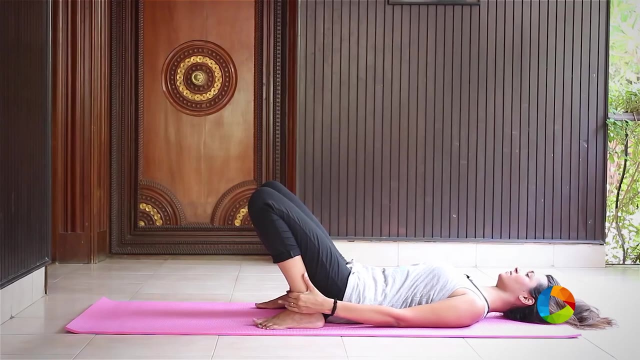 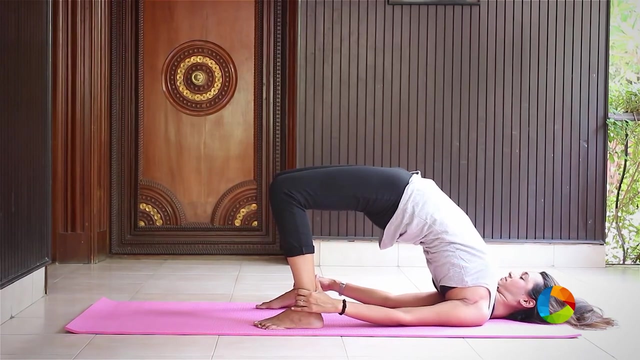 By combining the asana with synchronized breathing, your lung capacity can be improved greatly. You can also notice an instant kick in energy levels after performing this asana. Setu Bandhasana or Bridge Pose. This pose involves stretching and strengthening the neck, spinal column and chest. With regular practice, the asana can strengthen 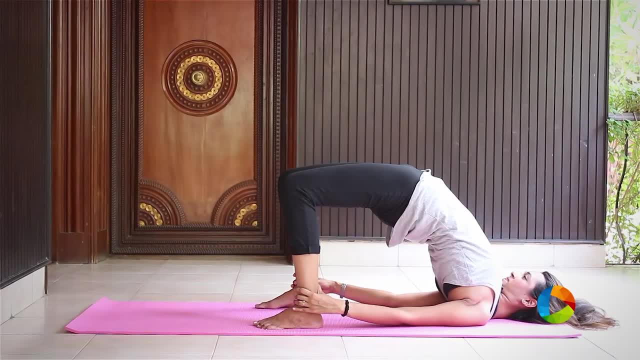 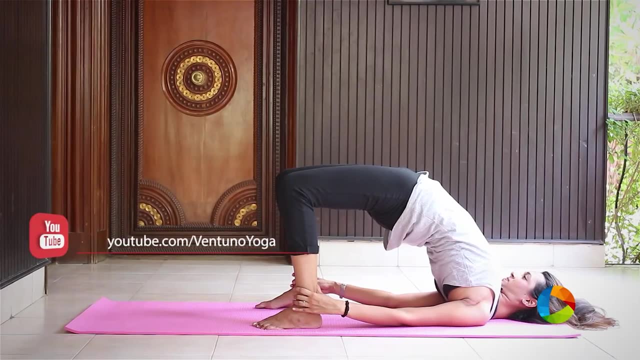 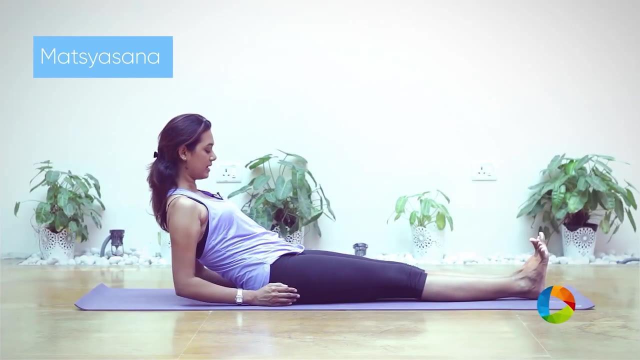 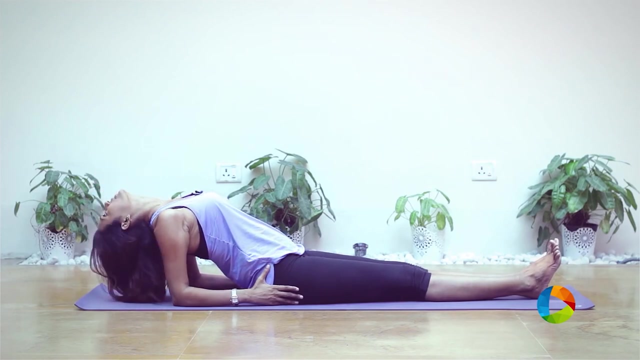 these parts and increase, along with increasing, blood circulation and digestion. Also, Setu Bandhasana can calm down your nervous system and alleviate feelings of depression, which negatively affects your immune system. Matsyasana, or Fish Pose: This pose helps in improving your respiratory tract and treats breathing problems like asthma. Holding this pose for about 10 seconds will.